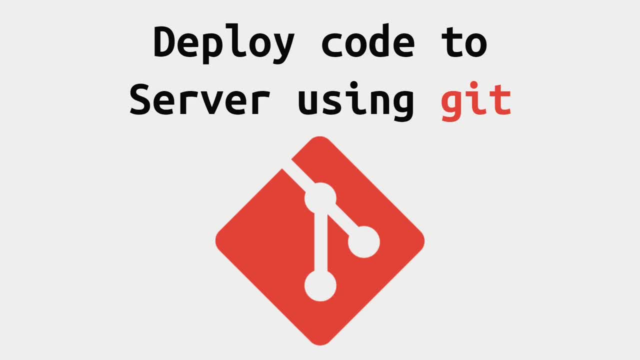 good idea. You just basically develop your code in your environment, in your home PC, and then connect to your server, and then you move the files using FTP to your server, which is like you zip it: you delete everything there, you move it and unzip. It's not a good practice. Maybe it works for one person, but if you 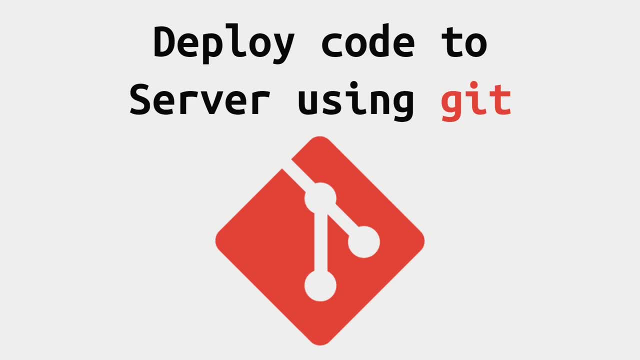 have multiple people. it's just not a good practice. Now you can use git to accomplish the same thing, which is a lot more safer because it does protect your code. You will not be able to rewrite your code. It's git, right. It's a version. 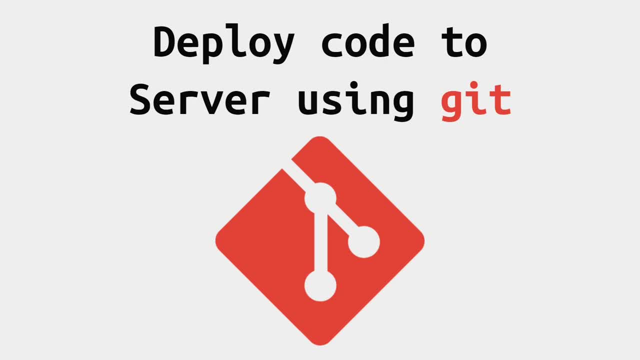 control. So if you accidentally delete the code or rewrite some part, it will tell you and you have to resolve conflict. so you will be safe in that way. There are a lot of ways to do this. actually, with git, There is what do they call it continuous development CD. 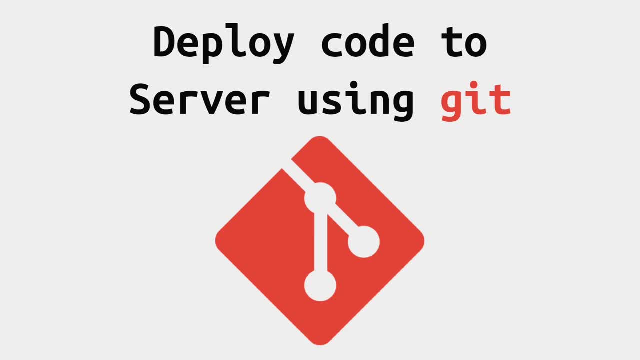 Those are for big companies. If you are a one-person developer, you don't really need to go through the hassle of setting up pipelines and whatnot for AWS, for git, all those things. You don't need that and this is going to be the way I. 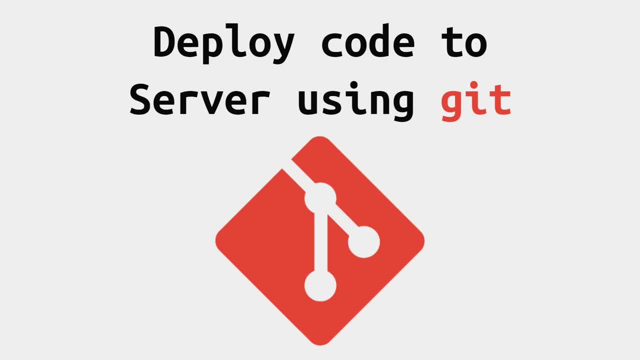 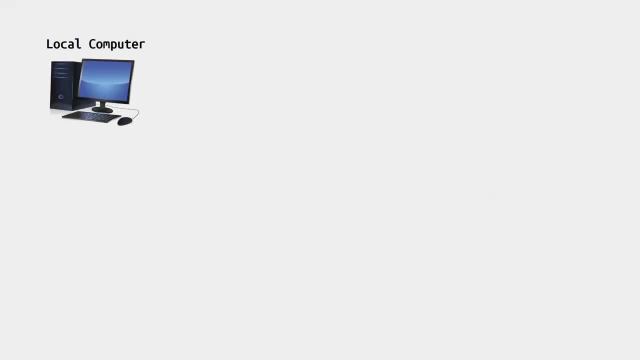 started Many years ago. it's very easy, very simple, yet effective. So let's see how it works. I just made a quick chart for you so I can represent the steps to you. Okay, on the left side we have the local computer. Okay, and here's my cursor: This: 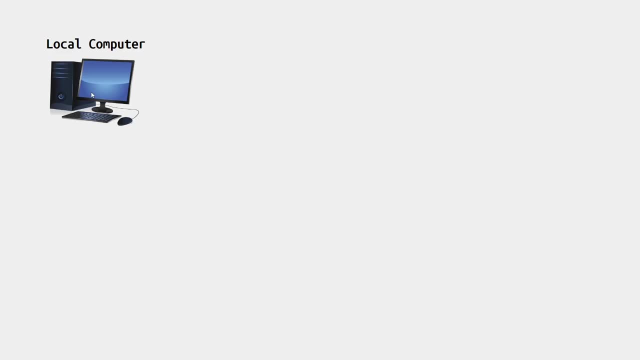 is your home computer. You're working, You make a code here. Let's say you make a website, indexhtml on your local computer, Then you add it to your git repository. Let's imagine you already made a git repository and you cloned it on your local environment. You add it and then 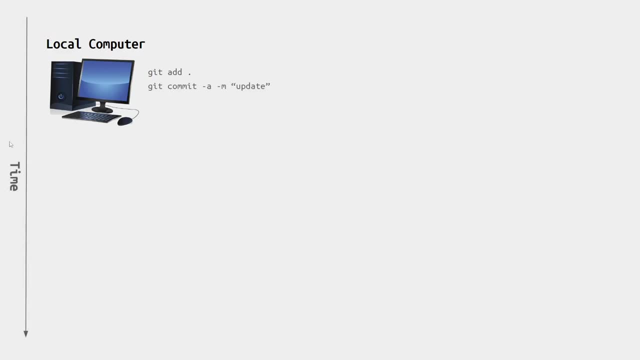 you commit the changes and then let's add this as a timeline. It's a step-by-step: This is one o'clock, This is two o'clock, Okay, this is a time downwards. and then you push it to the master and it goes to your git. I 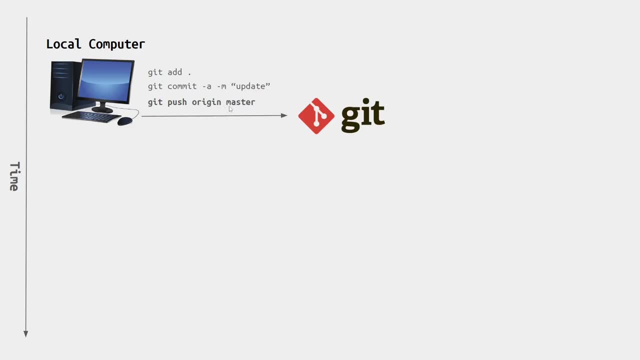 mean it changed to main. Now git push origin main is just a bad habit of mine. I keep writing master, So you push it to git. Now you simply you have to go to your server and you have to SSH to your server and I'm going to show you an. 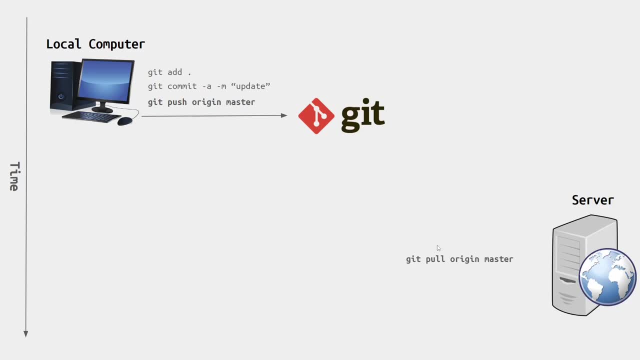 example, And then on your server, you clone the git repository. Once everything is set up- which is very easy- then you pull the git from the origin main or master and voila, you'll have the code working there. It's that easy. So let's. 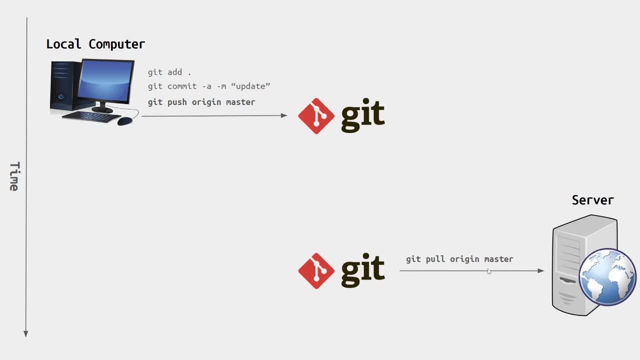 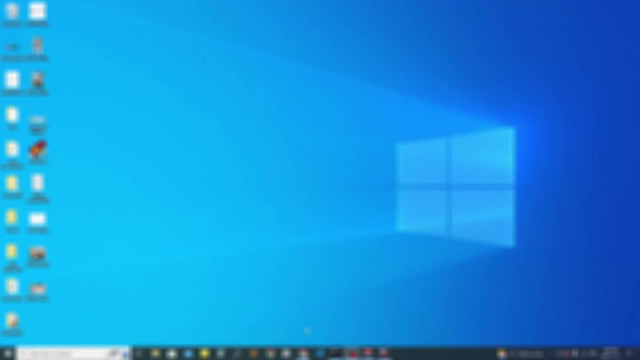 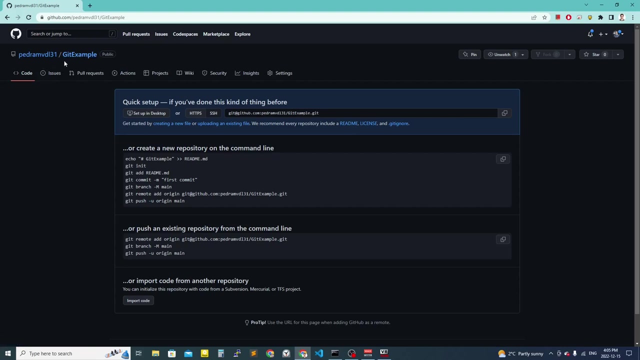 get to it. Let's actually go, and I'm going to show you a quick example. All right, see how it's done. All right, so this is my home computer. This is my. I made a repository in my github, calling it git example. All right, so the first thing you want to do, 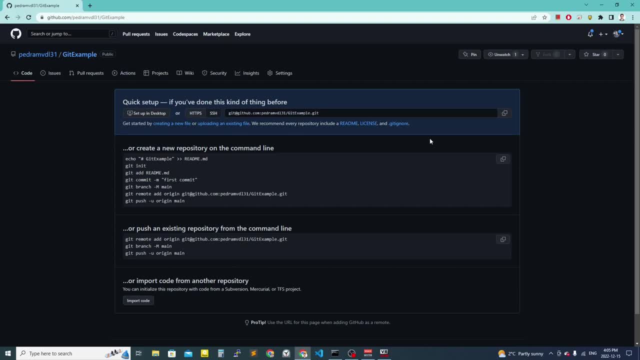 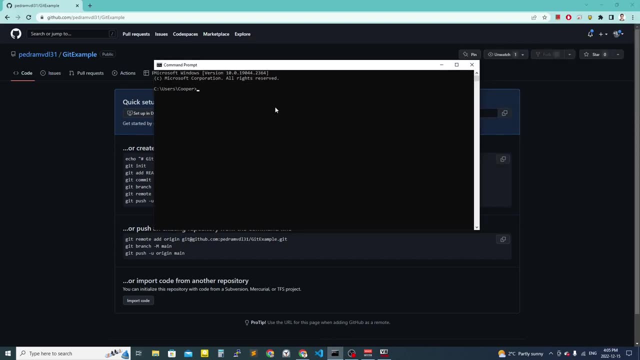 you want to copy this- and I'm not going to talk about SSH keys, because you need to add those things to be able to pull- and and then I'm going to go to here, I'm going to go to my coding folder and then I'm going to say: git clone. 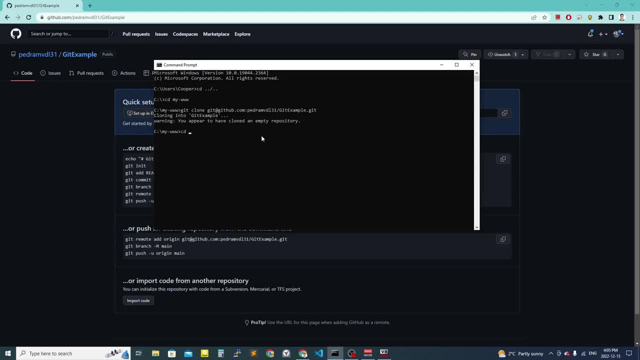 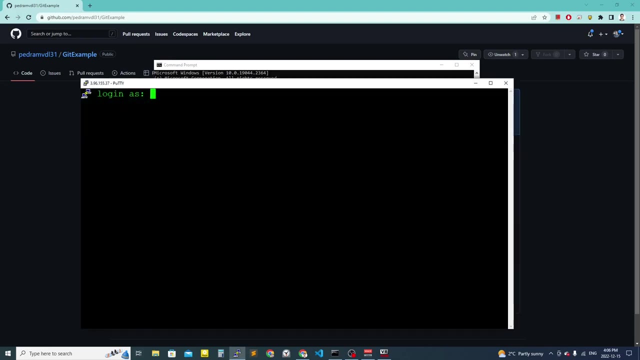 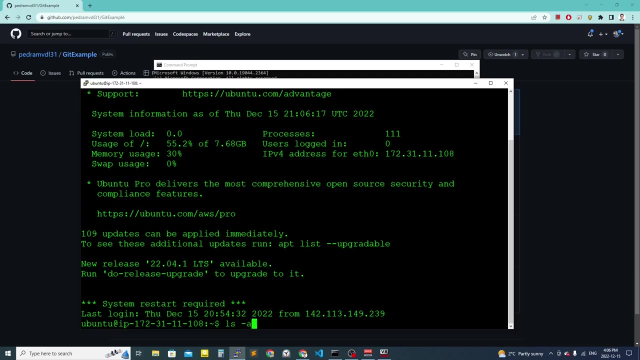 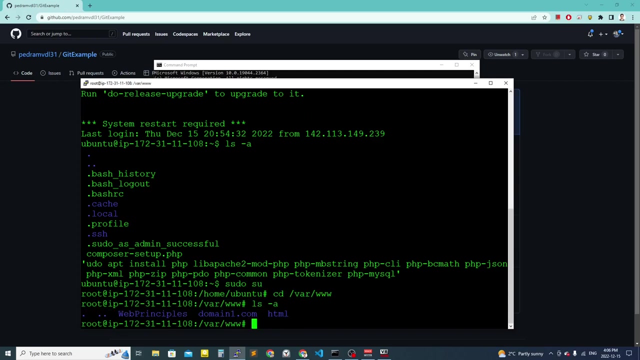 is GitHub. Alright, very good, Very nice. Now what we want to do is we're going to All right is to use potty and go to SSH to our server. I made this using AWS, so it is online, all right, where are we? okay, so we are here. I already added couple of routes, so 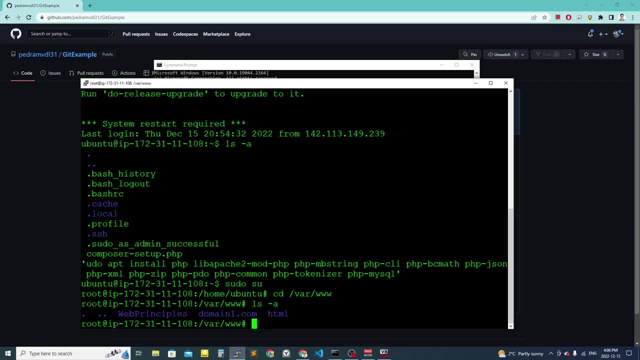 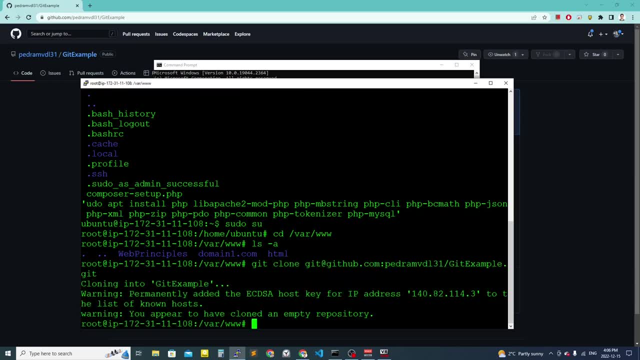 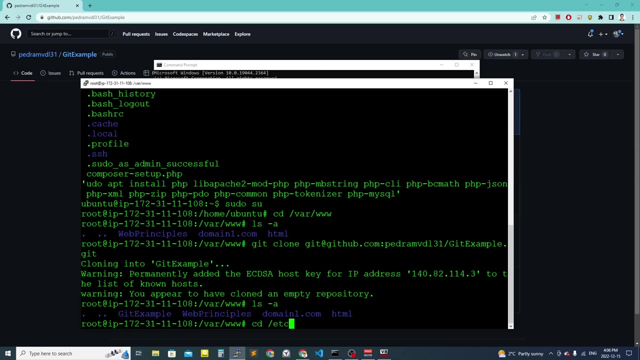 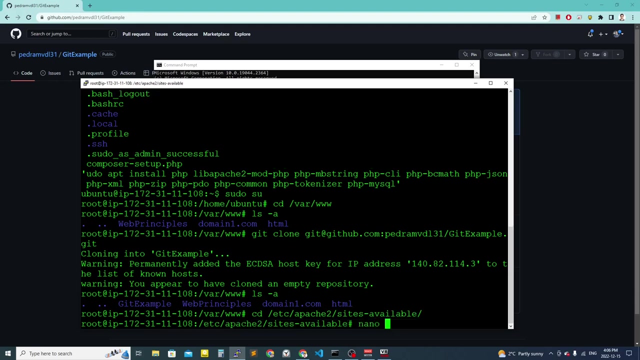 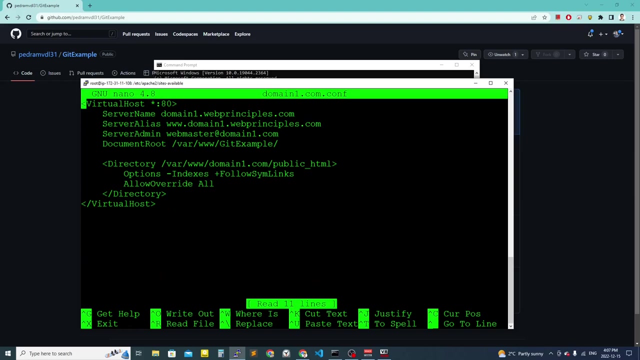 that it works. let's first do the git clone and the SSH keys added too, so I'm adding the same repository here. perfect, let's go see if I set the Apache properly. you perfect, it goes to that folder. I already did that just to make sure this video. 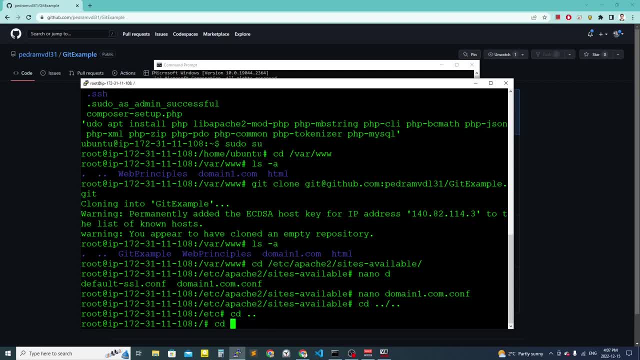 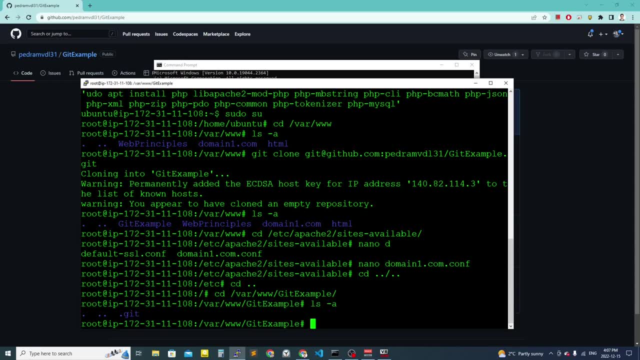 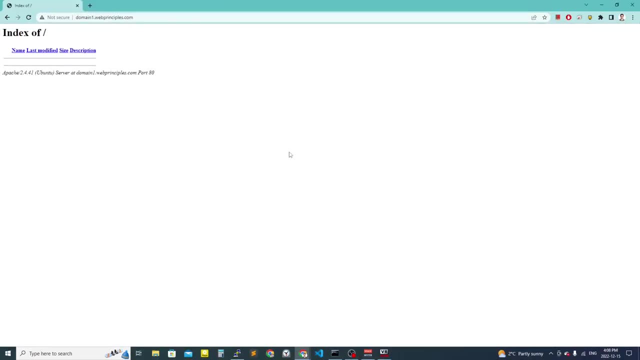 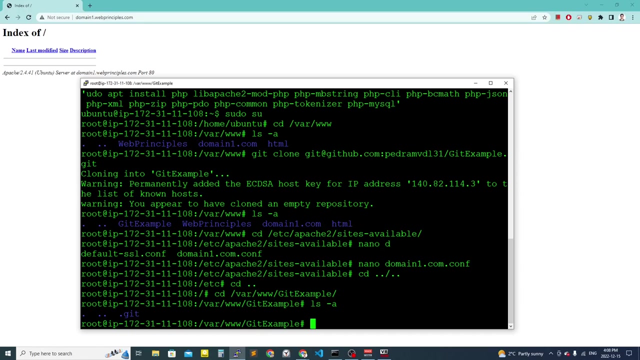 actually actually talks about the things that you guys want to hear. and let's go to the folder, right? so we are inside that empty folder. I'm going to open that subdomain that I set, all right, so this is where we are. I'm going to test that quickly, just for you, for your information. 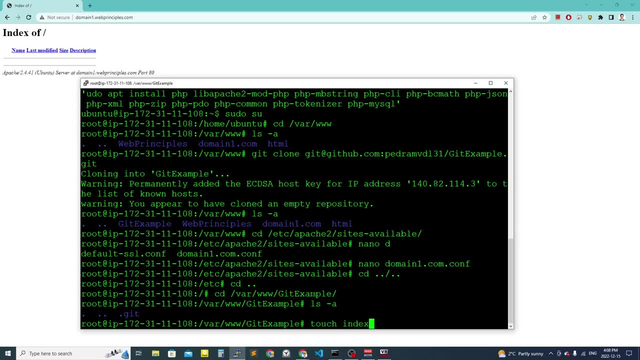 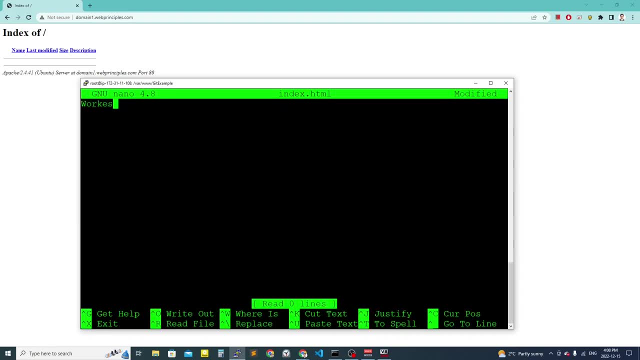 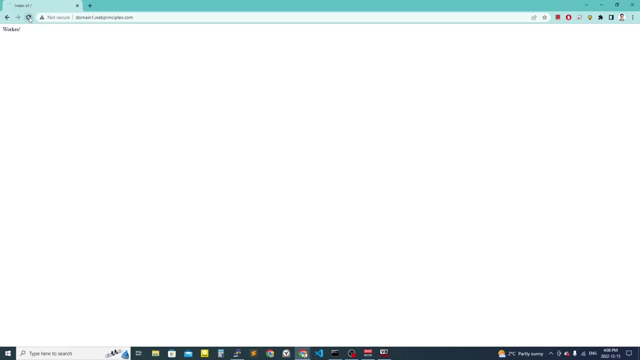 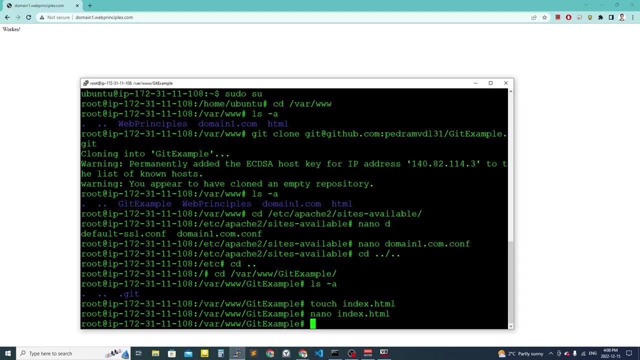 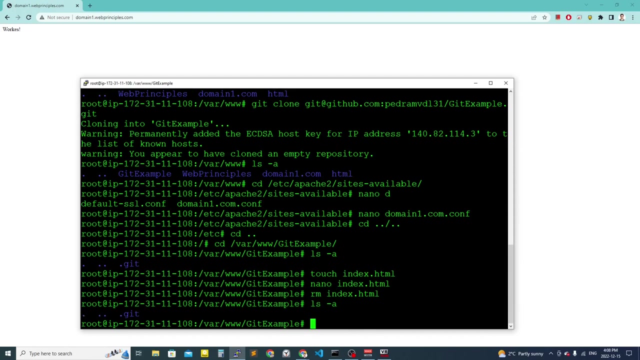 so let's do. what is it? touch index, dot, HTML, nano index. let's say works, save it and then reload. perfect, so we're keys, so that works. let me delete this all right now. the whole point of this tutorial is to develop on your local environment and 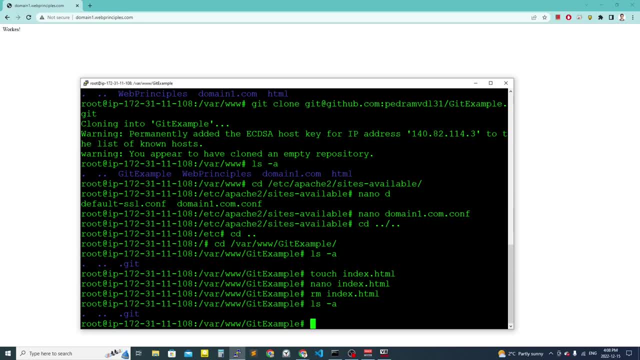 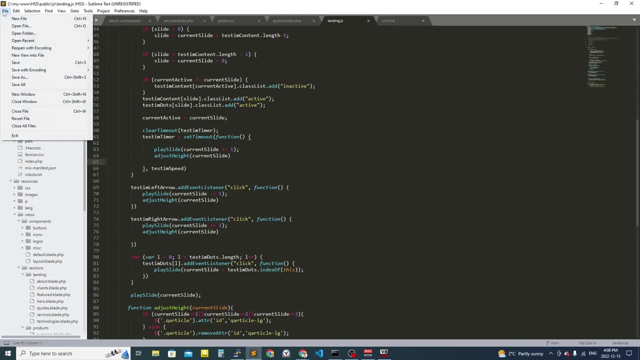 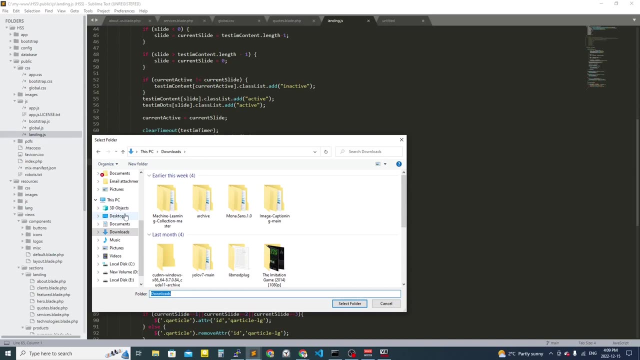 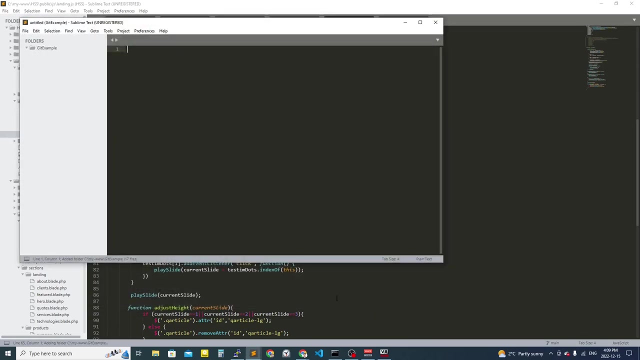 then move it to the gates and move it to the server without having a hassle of FTP and whatnot. so open your favorites code editor, open the folder that you once- and it's going to be in my see- here you and this one. perfect, there you go. 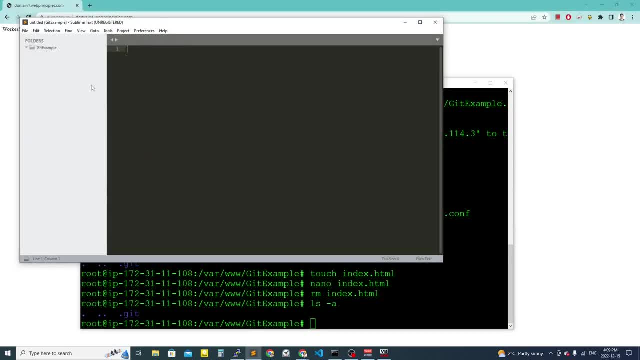 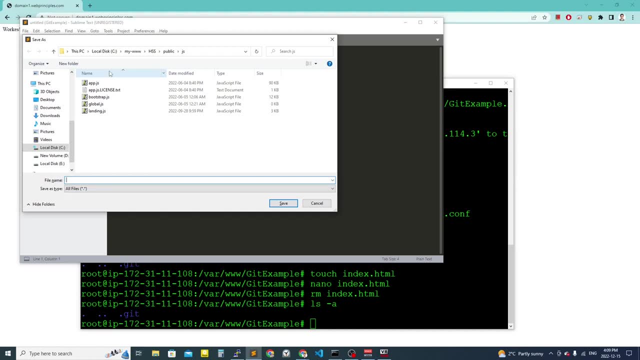 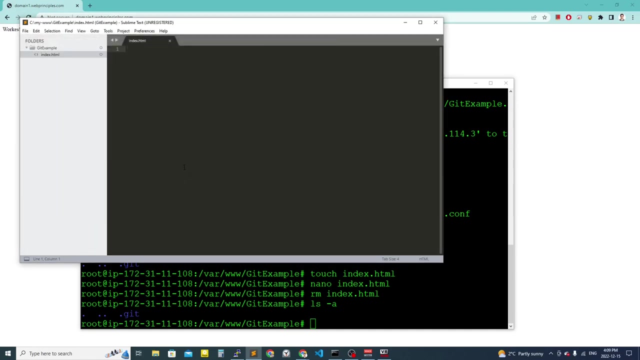 it works. so in here we add: it's our local environment. again, I hope I'm not speaking too fast. grace we are going to save in this dummy should remember the location. let's say index dot HTML. okay, let's add a. see, here we are going to add a. 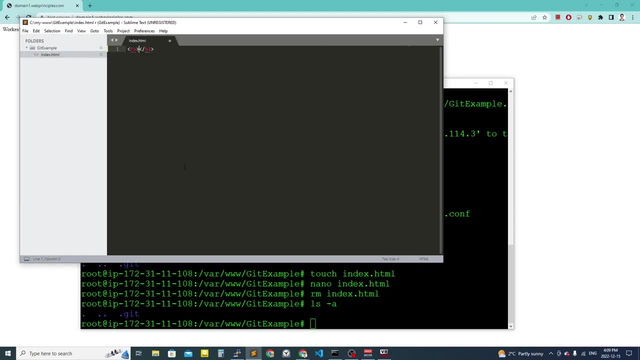 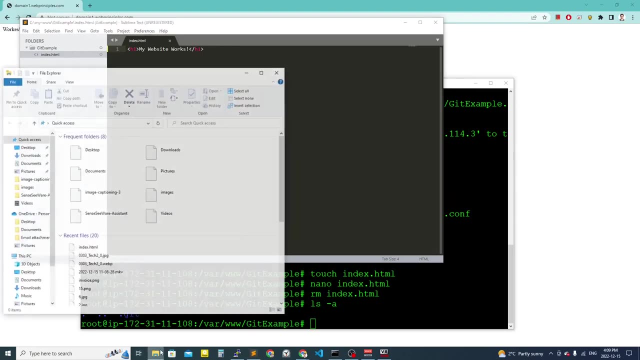 title link format and a subtitle if we are going to add the talvez content, a subtitle message if we are going to add, and one that we can then select it. so either a budget or not. okay, it's the canvas, this hygge, dashboard, jobs, same thing. okay. so you wanna make sure you edit. 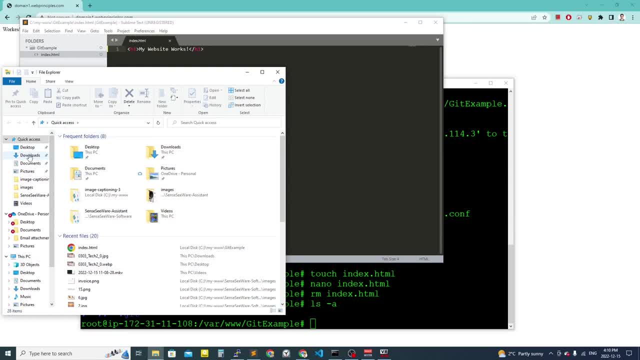 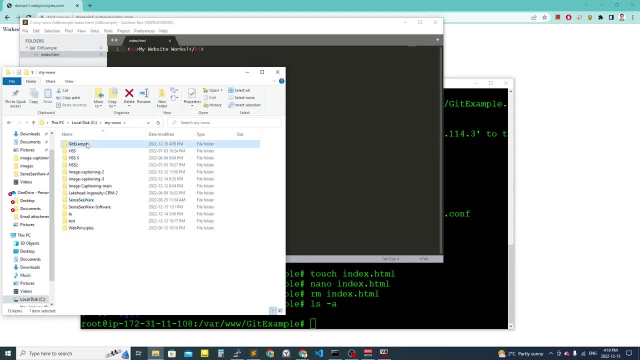 your website by make sure that you're not on your website or you are using a mind job website yourself. if you have aatable website to update, searching open website- awesome. so we are going to do this here. for example, go to thinkorg, then click where your website's located, then click update. 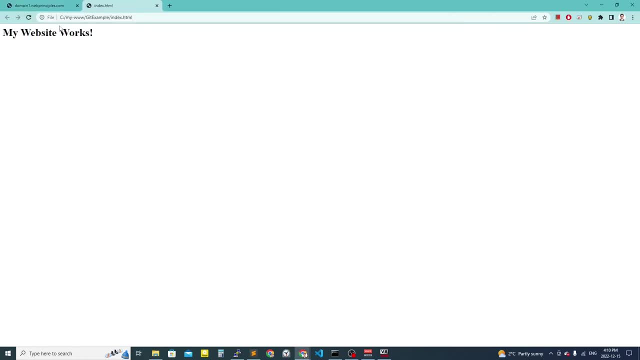 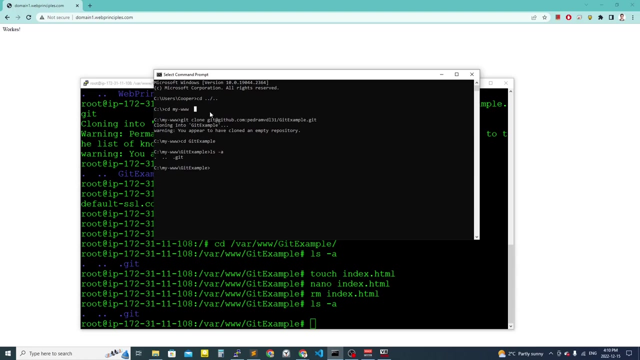 w kids can just open it from here. my website work and it's in. see my w w w. okay, let's close this. now we want to move this to the server, right? so this is my local cmd local command prompt. so here, very simple, git add. i'm adding the whole thing. let's see the git status. 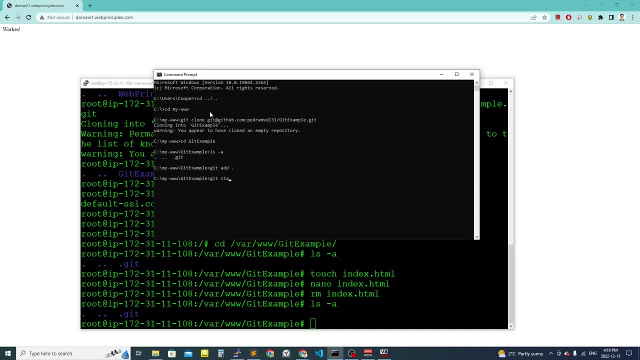 oh, my g button is not the best git status, so we added the index file and then git gets commits a, a message. let's say: init initial, push perfect and then git push origin. what's main voila? that's it. so now this information is in git. it's not on the server yet. 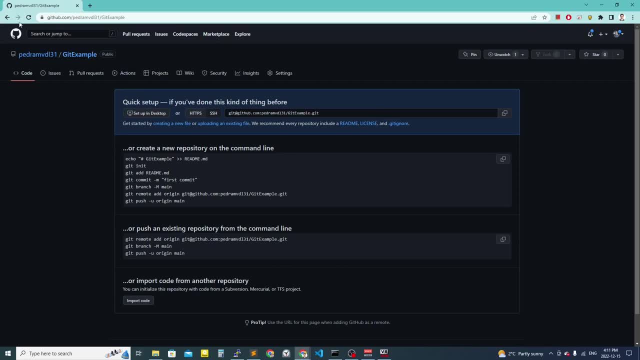 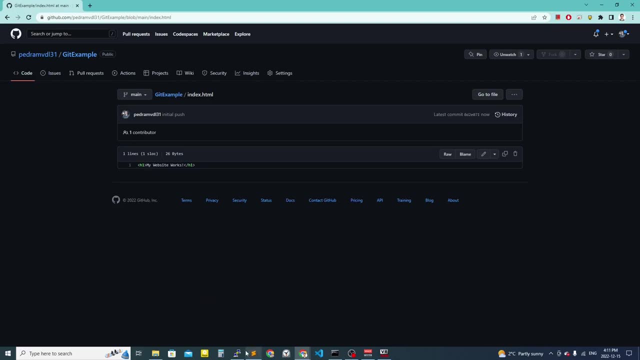 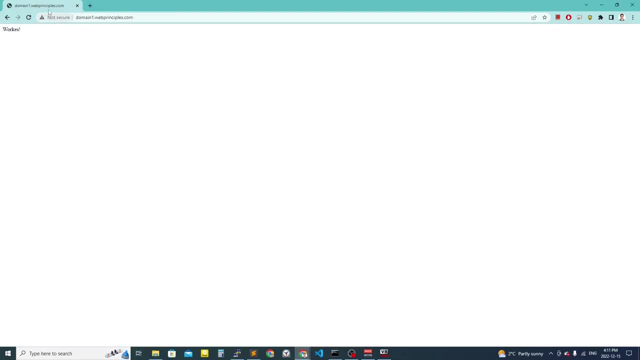 right. so if i go to our repository and if i reload this page, the index file is here, right? very easy. now i will go to my server and let's even look at the, the domain itself. so i'm going to go to my server and let's see what i have here. 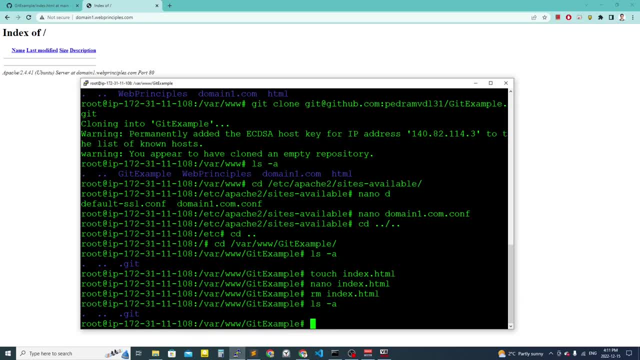 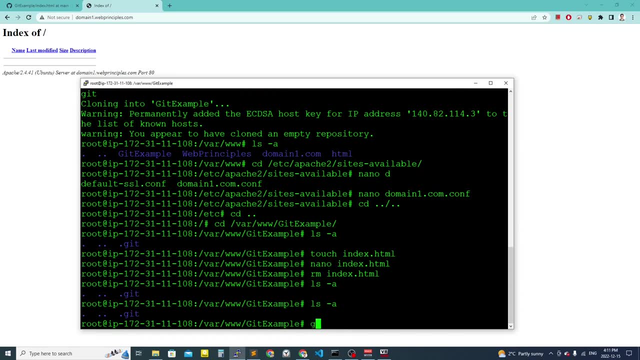 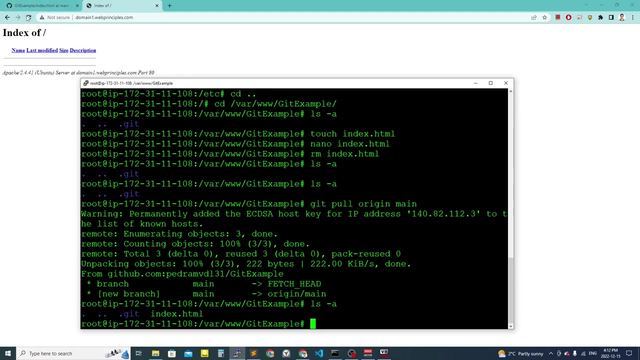 obviously it's not there yet because i deleted that file. so now let's go there. and this is my ssh potty, that's lsa. there is nothing there. i can do git pool, just like the diagram. i'll show you git pool: origin main: perfect. let's see what we have. the index is there if i reload. perfect, see, that's it. so i'm going to. 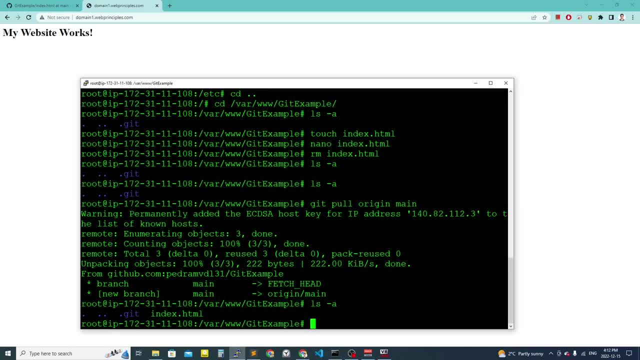 call it the best file, right? so i'm going to say dot, git and it'll do it for me and i'm going to have a file that i want. so now the beauty of this is obviously, i made only one index file and it worked. it will work for anything. you can have thousands of files and you can have 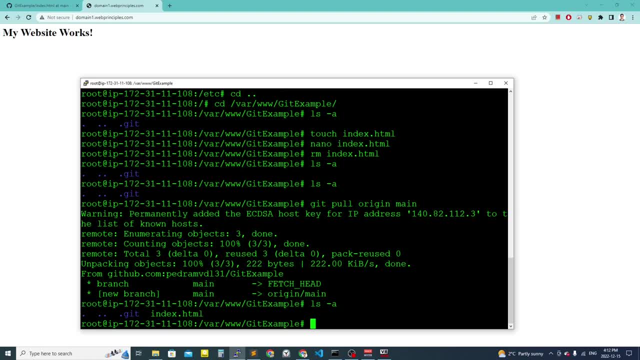 hundreds of developers working on this project and they all push everything to the git and one person, who is usually the project manager, will check the code and then pull it. small team, I really don't see it as it to be necessary. well, I guess that is it.